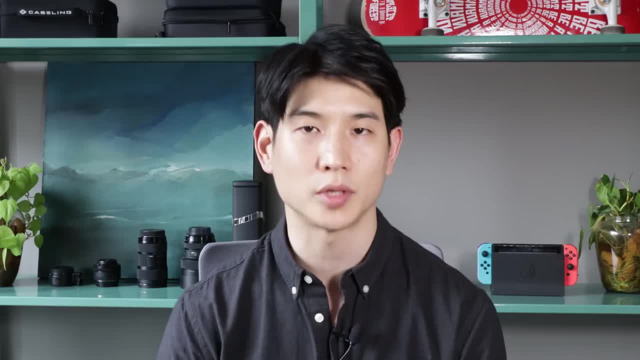 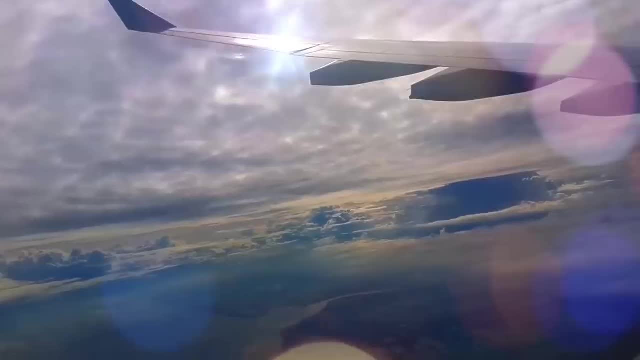 At this point, though, already I was starting to love the journey. I really liked problem solving and I could see myself doing something like this long term. So I did what any sane person would do and I quit my job and I moved to Korea to minimize my expenses and I decided to learn full-time. 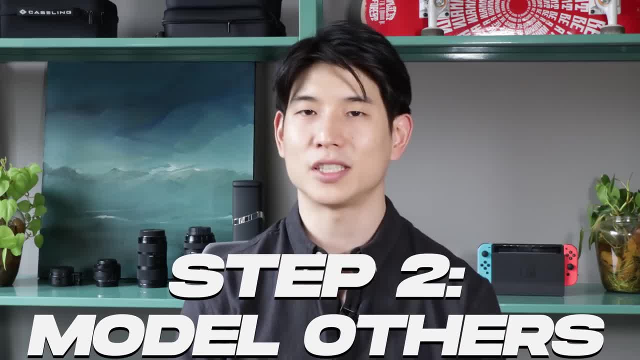 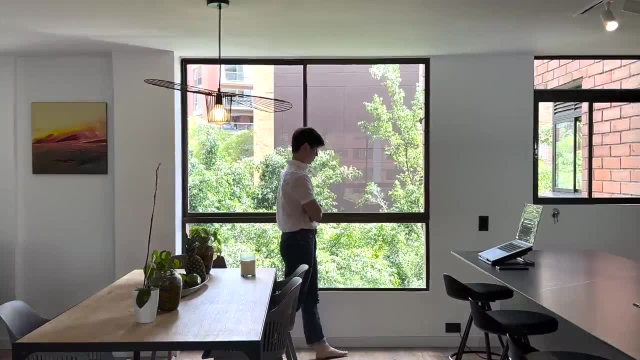 Learning full-time was a lot harder than I thought. I've actually never studied anything this complicated or tough before, and I was quickly starting to realize that I didn't really know how to study at this pace. I would sit in front of my computer and hours and hours would go by. That was 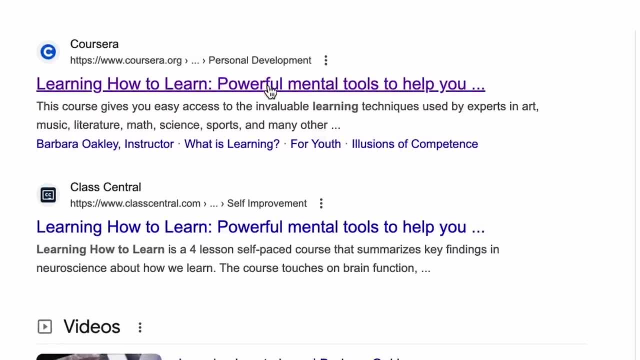 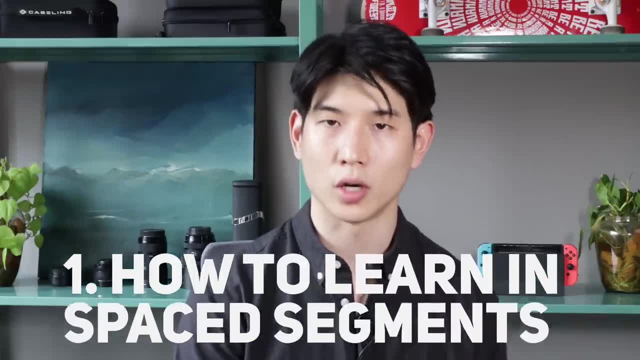 when I found out that there was a course called Learning How to Learn by Barbara Oakley. This course was life-changing. My two main takeaways were one: it taught me how to learn in space segments, a technique called Pomodoros, and the course taught me that I needed to create a dedicated 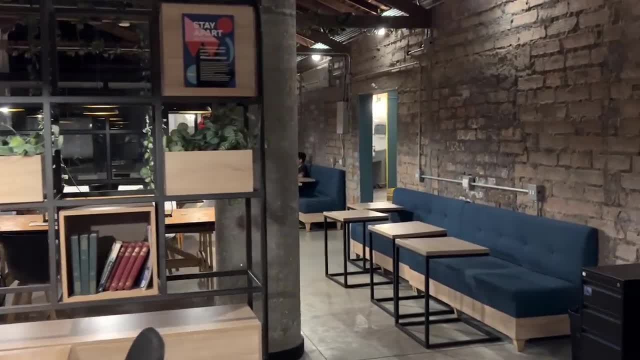 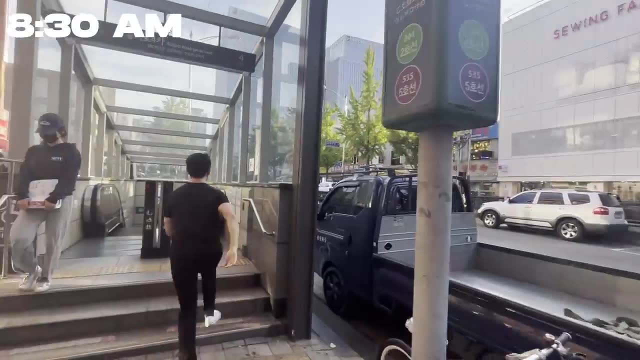 space for learning. So I joined a co-working space so I could focus better. Now, armed with new knowledge, I got back to studying, and it worked. Here's what a normal day looked like: 8 am- Wake up- 8.30.. Head to the train station. 9 am: Arrive at the co-working 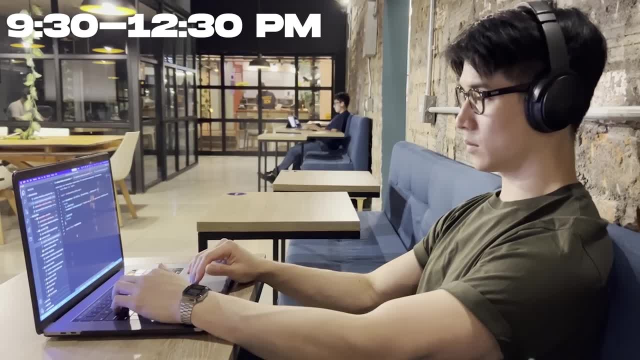 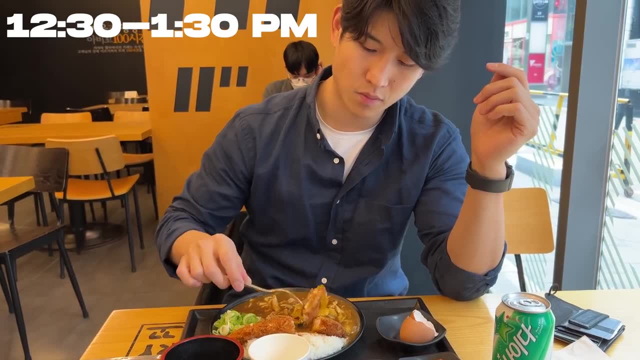 space 9.15.. Coffee, Journaling, Reviewing the curriculum: 9.30 to 12.30.. I would have my first study session where I did 30-minute increments of Pomodoros From 12.30 to 1.30, I would eat. 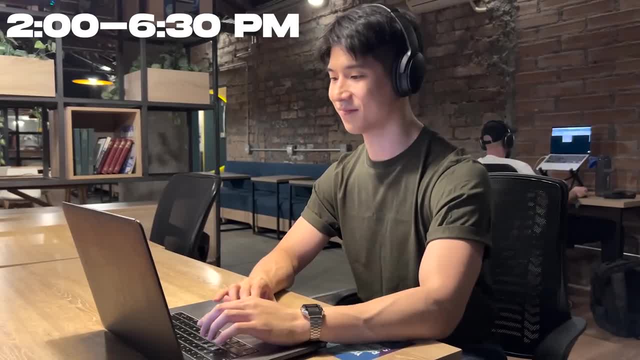 lunch and take a small break. Then back to studying. From 2 pm to 6.30, it was more 30-minute increments of Pomodoros until I was ready to head out. From 6.30 to 7.30, I would gym. 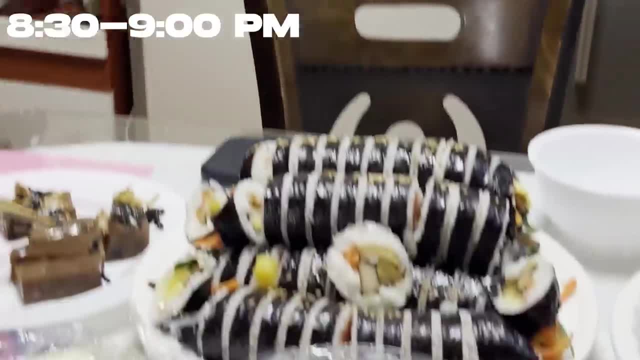 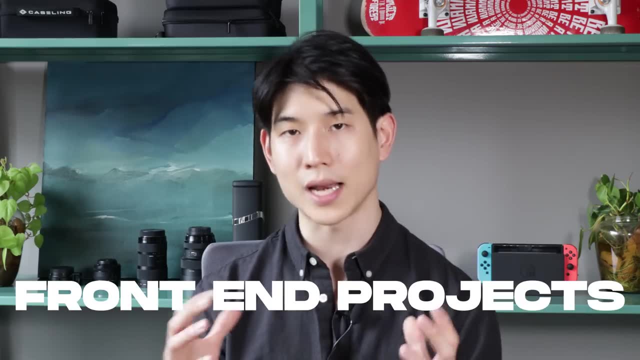 three times a week And then 8.30 to 9, I would eat dinner with my grandma, then help her clean. This was my schedule for six days a week, no exceptions. The next part of free co-camp was a challenging Front-end projects. They essentially give you a list of projects that you have to build. 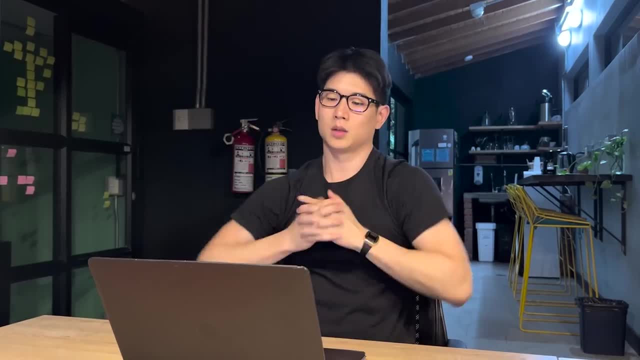 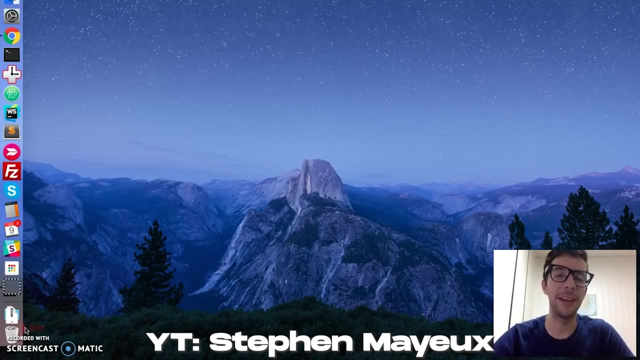 using HTML, CSS and JavaScript. To me, this felt like a massive jump, because I never actually built anything before. I felt stuck at this stage until I found a YouTube channel of this guy named Steven, who would stream himself building these projects line by line, By copying him and recreating what 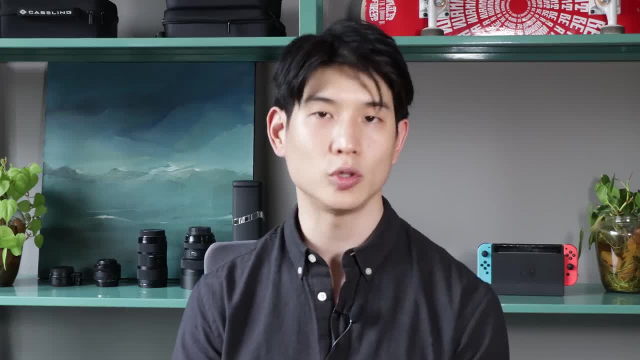 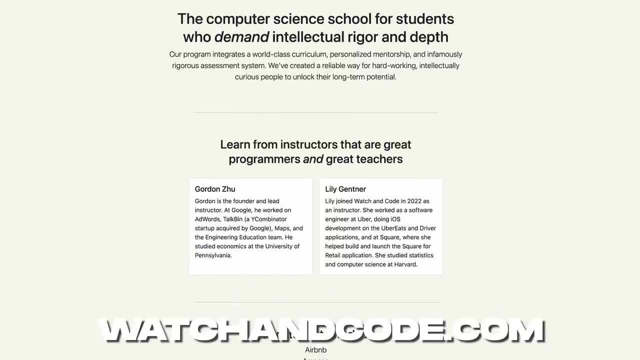 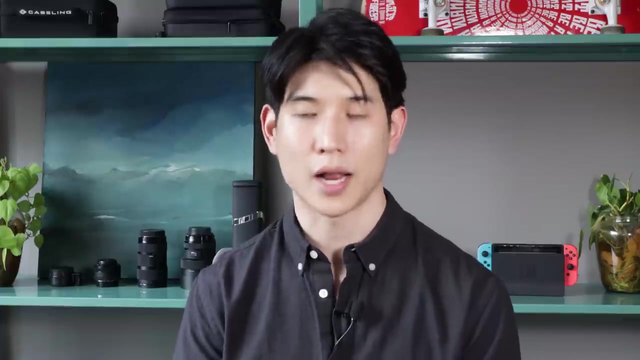 he was doing. I was able to use that experience and build the next couple of projects on my own. I also found a great resource called Watching Codecom, where you watch and code By following along once again and modeling others. the concepts really started to take hold And I was really starting to understand what I was doing, not just 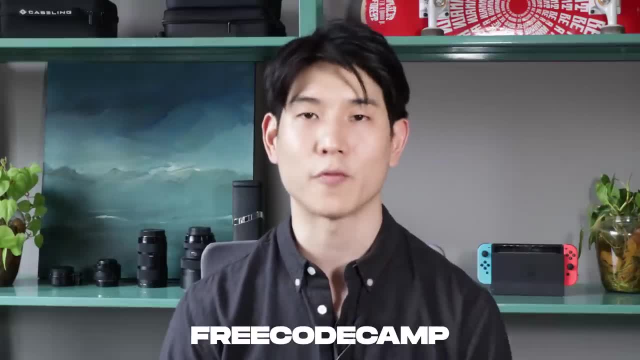 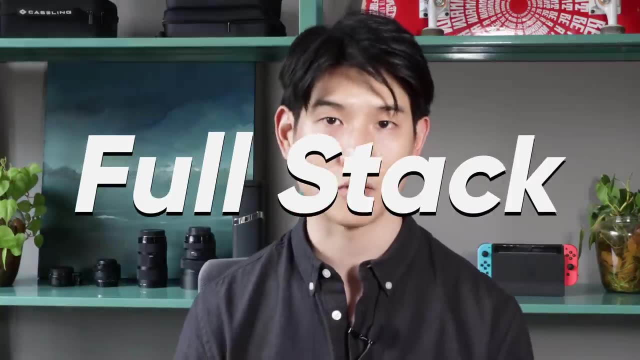 solving a math problem. In exactly one month, I ended up earning my free co-camp front-end developer certificate. I was learning a lot, but I never actually built anything full stack before. Something with a front-end or an interface, the thing that you see within the browser, a database where all 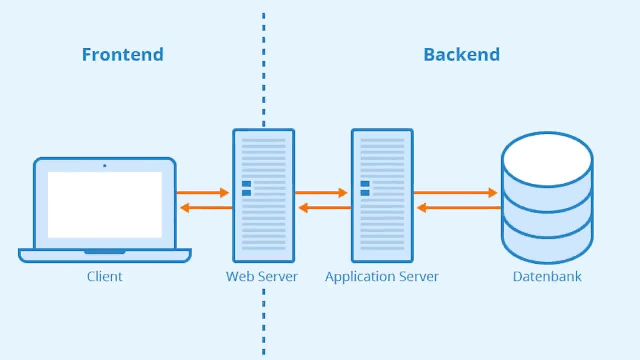 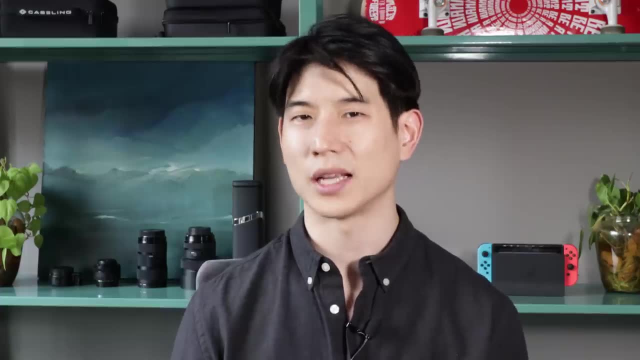 the data is essentially, and a server which handles and manipulates all the data in the back-end by taking in requests from the front-end. So I still felt like an imposter and not a real developer. You're not an intellectual, You're a fake and a fraud. 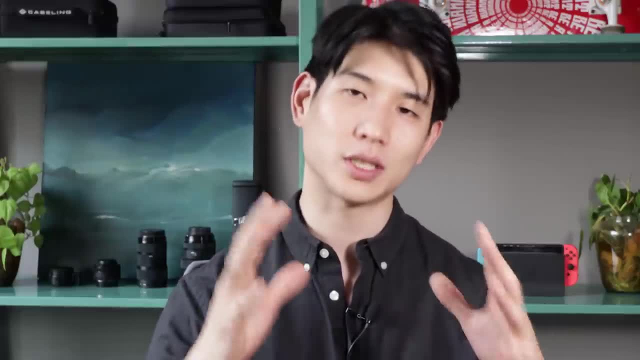 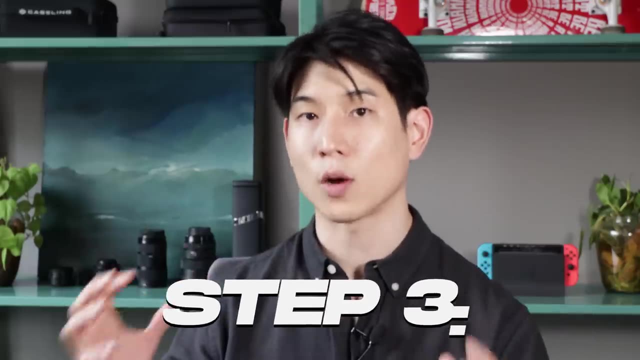 So, to become a programmer, I decided to build my first full-stack project. Remember Steve with the YouTube channel. I reached out to him to get his assistance, to help me build my first full-stack web app. We decided to meet three times a week. Here's what we did. We picked one major project. We tried to use my first full-stack website. We decided to have a live meeting with Steve. He decided to take all of his time and video and have a short one that had no text. I tried to make a video and it was super random. We. 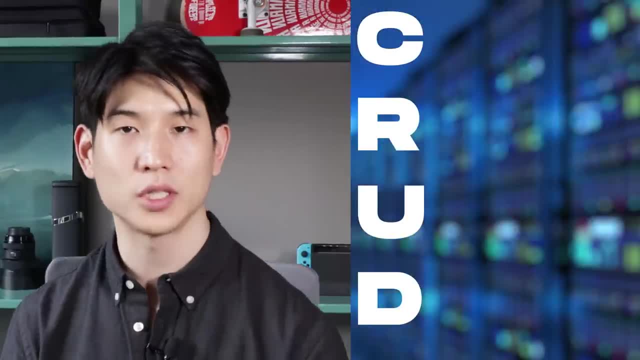 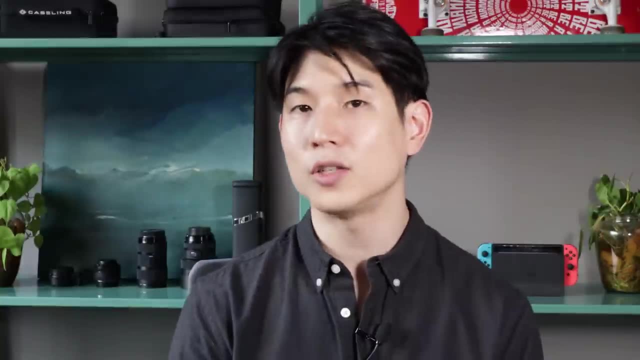 major overarching project which will teach me the basics of CRUD, which is create, read, update and delete. These are the foundations for any web application. I decided to clone Pinterest. I honestly don't think I would have gotten a job without this next part, so pay attention. I asked. 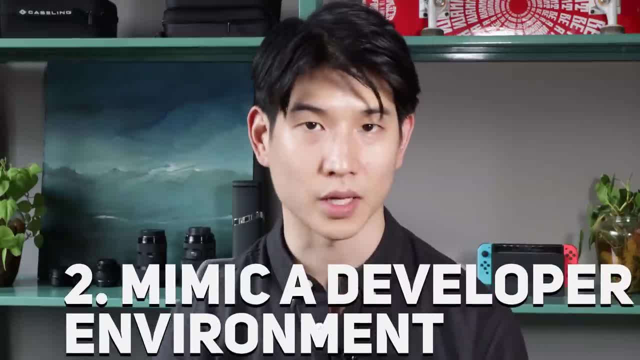 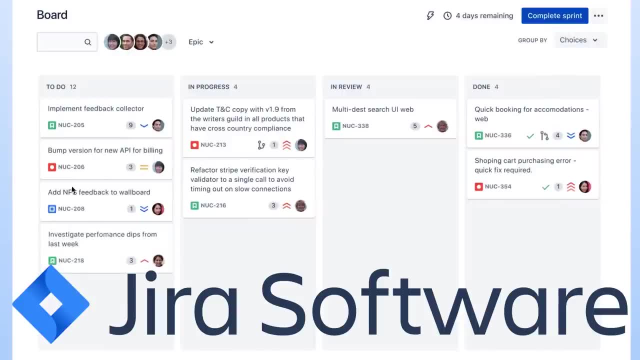 Steve to treat me like a real junior developer working at a company. We implemented a project management tool called Jira. Use Jira to compartmentalize the entire project and write the requirements of exactly what I'd be building. This taught me how to estimate my work and plan. 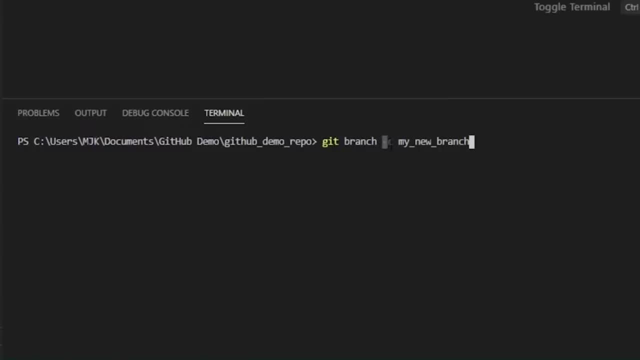 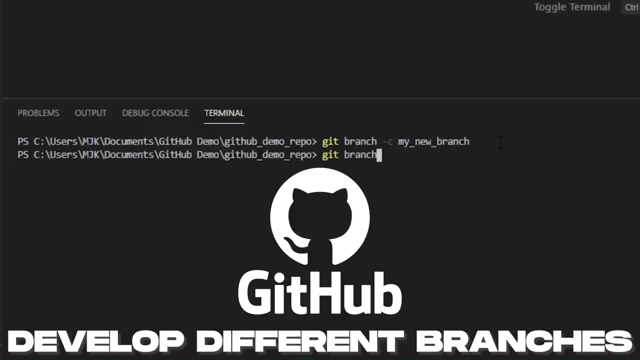 how to build an entire web app from zero to launch. We also set the project up on GitHub, which is a version control application. This taught me how to develop different branches for when I was working on certain features and I could learn how to control different versions. 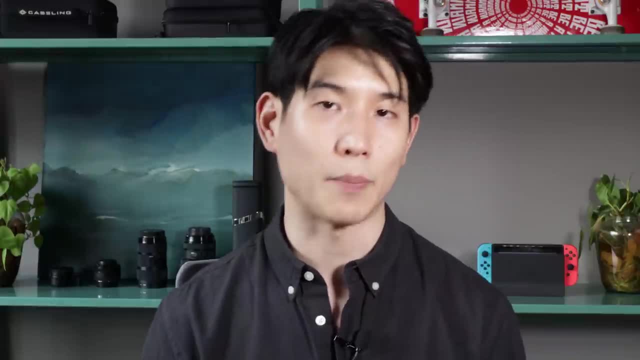 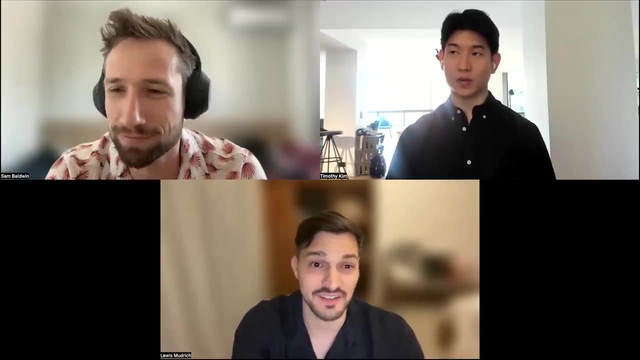 of the code. Most tech companies use some version of the two applications, because being a developer isn't just about knowing how to code. it's about knowing how to work collaboratively with other people as well. Steve grilled me on our pair of programming sessions. He was very strict about me keeping 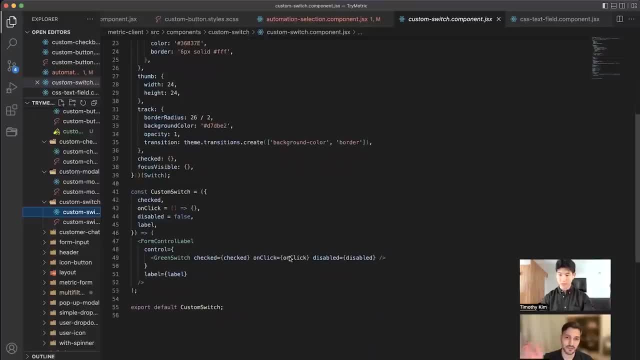 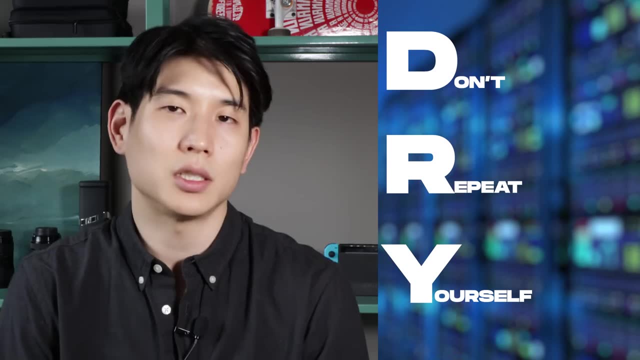 the deadlines and the estimates that I originally wrote out for myself. He would constantly question why I was doing what I was doing, and he even taught me the concept of DRY- just don't repeat yourself- or, essentially, just making reusable code. I had to learn how to build by googling. 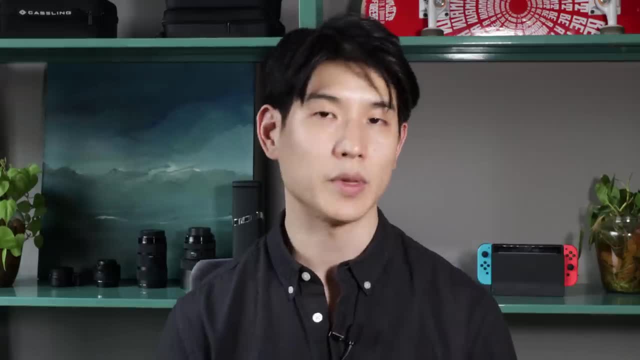 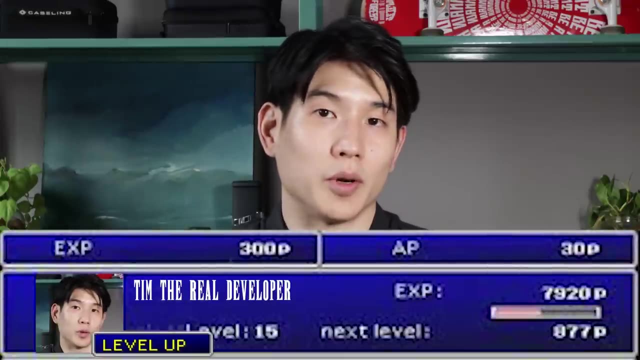 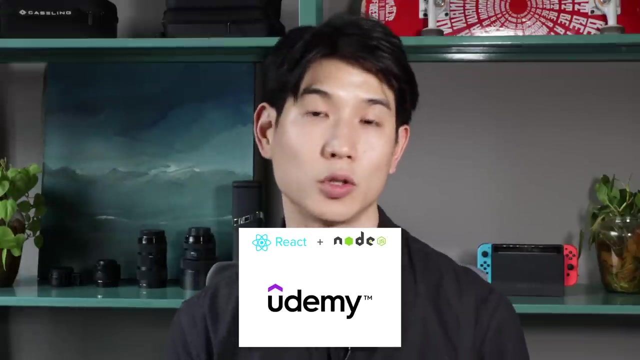 for answers and using sites like Stack Overflow, and he would leave me a lot of comments on things that I needed to change, so I learned how to debug my code on my own. This made me feel like I was a real developer. Over time, I supplemented my learning journey with Udemy courses on React and Node, because these 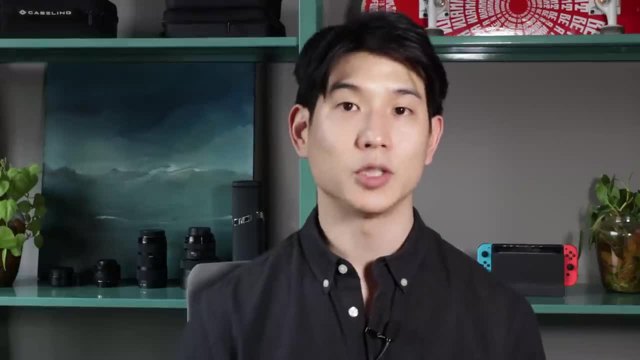 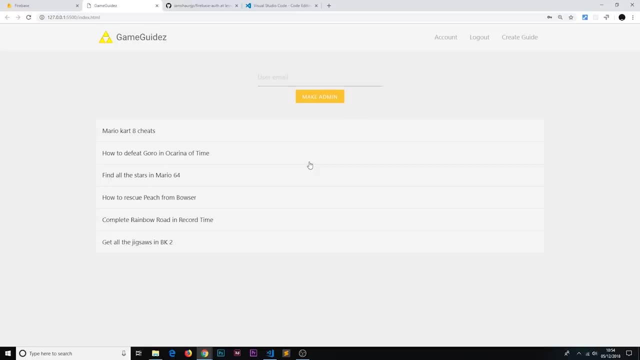 are the two frameworks that I chose to build my Pinterest clone. As a result of building my first full-stack project, I ended up learning how to do things like how to design a database, build APIs, set up auth and eventually push the app to a cloud server. These are all things I would have. 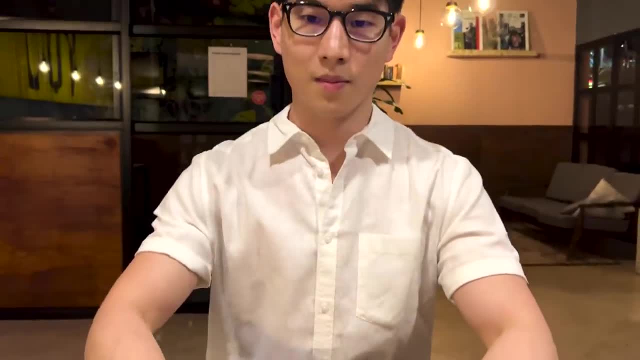 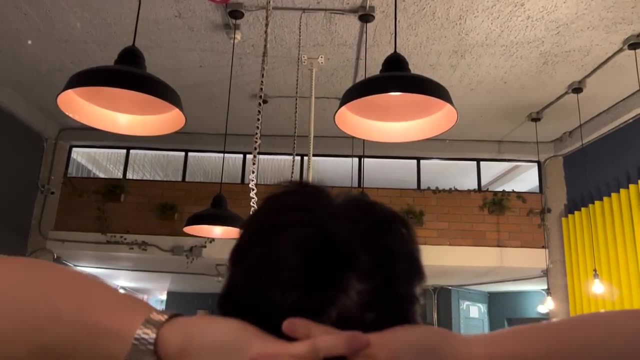 never learned by just doing tutorials And in around two months I finished my first full-stack web app. I remember when I finished the app I felt like a real programmer. That's when reality set in and I realized I'm still broke. I haven't made a single penny in over. 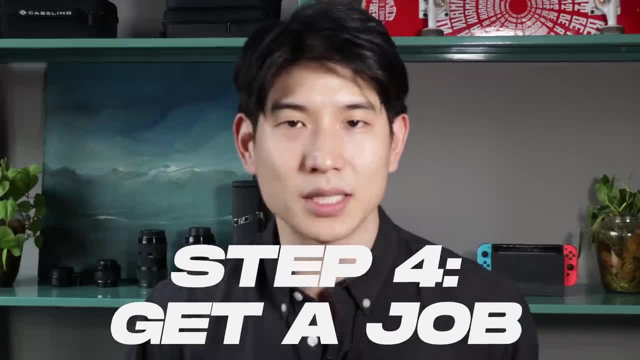 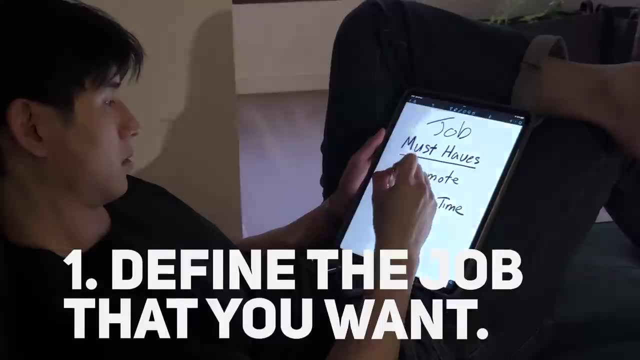 a couple of months and I still needed to find a job. It was time to see if everything that I learned was actually worth anything. First, I defined the job that I wanted. I wanted it to be remote and, most importantly, I wanted to work for a small to medium-sized company, because I hate working in a 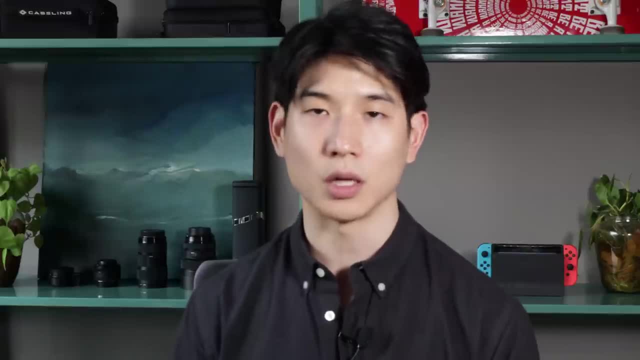 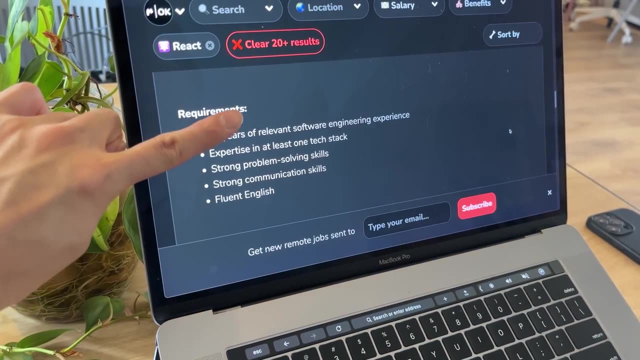 corporate environment. I found all the jobs that fit my parameters on sites like WeWorkRemotelycom and RemoteOKio And, instead of just working in a corporate environment, I found a job that fit my just applying to these jobs. I found the contact information of the hiring managers and developers. 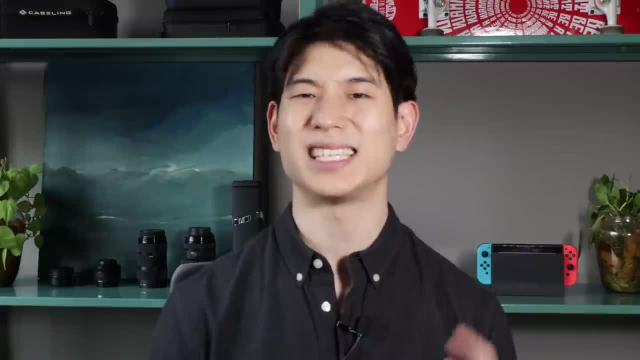 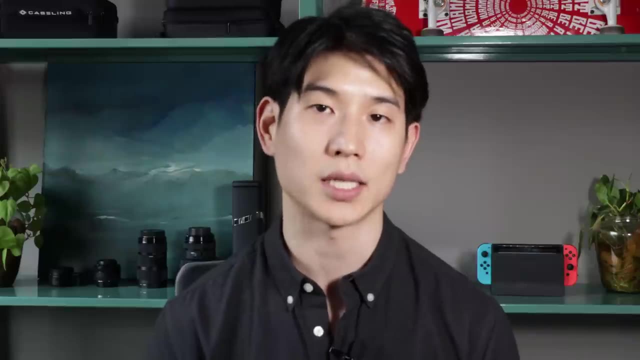 who worked at the company and I messaged them to introduce myself. I explained exactly what I had learned up until this point, what I was looking for. I even included the link to my GitHub so they could see the products that I had built. Most importantly, I included an offer that I know.